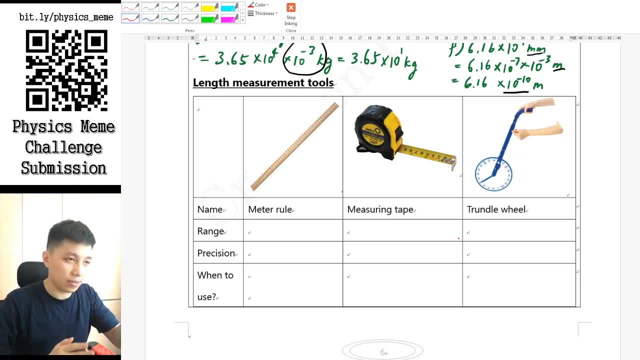 measure length. I will do the one on the left as an example and I'll leave the other two for you as a practice and then we'll discuss so. for the first one is called the meter ruler, which I'm pretty sure you have seen it in junior science, for its range is referring to how far. the maximum that 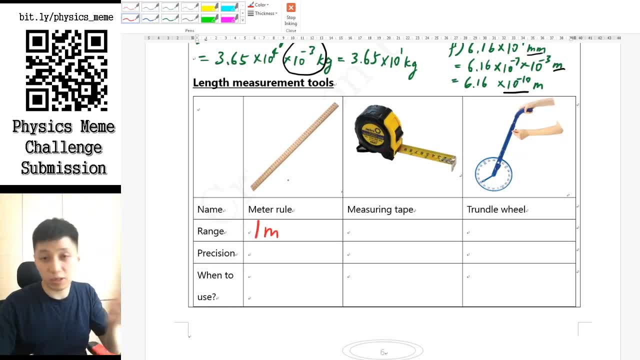 it can measure up to, so obviously it is one meter and that's why I call me. it's called meter ruler for precision, in case you don't know what it means by precision. that means the smallest distance you can measure up to, so it's like in between the marking. 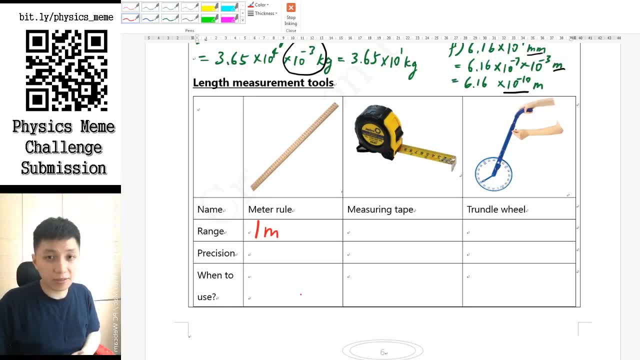 how far it is for the smallest distance. so in a more professional or more standardized way of saying, in physics this is called the smallest division or smallest graduation. so I don't have a meter rule at home, but then I have a normal rule. I just randomly grab and so if you try to 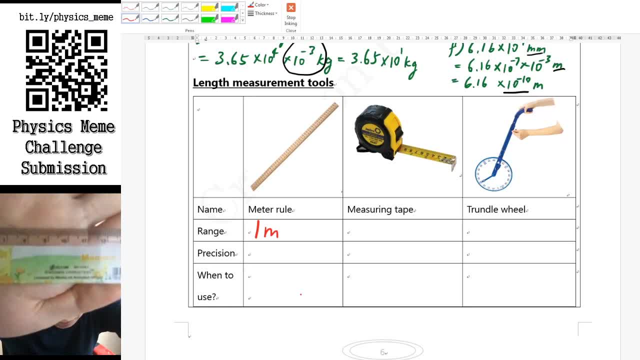 pay attention to that you can. you can see that this is in one cm between a number and there are 10 division between them or 10 interval between them. so that means you can measure up to the smallest distance you can measure, the smallest distance you can measure. 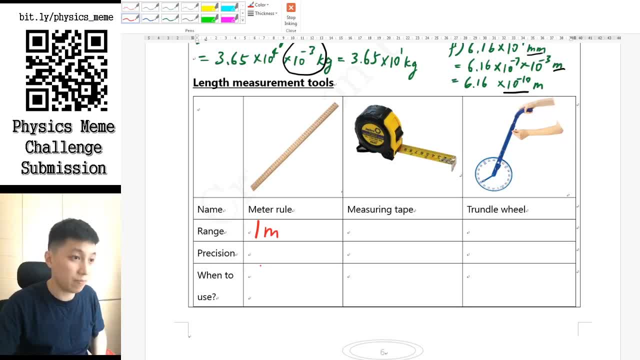 each interval will be 0.1 cm. I'm pretty sure that this is the same for most of the meter ruler that you can find in the lab, so I always call this 0.1 cm. as for the precision, it also means that whenever you measure something, the best you can measure is up to this, only up to a, this decimal place. 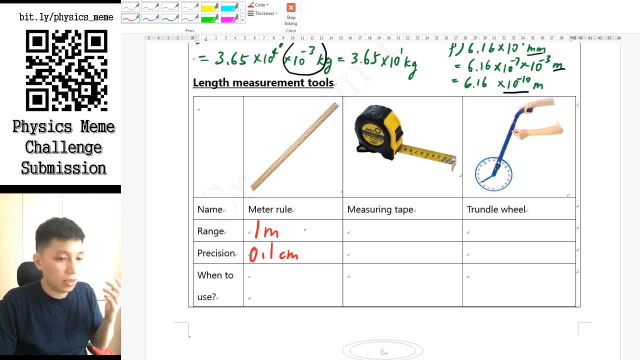 only so. for example, if, say, I have got a, a, say a USB or a drive or something like that, I can measure that distance. what would I do? so if I have a Taylor drive? you want to, you want to measure it. the best I can measure is probably, if I try to do it right now, it's about 6.7, ok, 6.7 cm, but 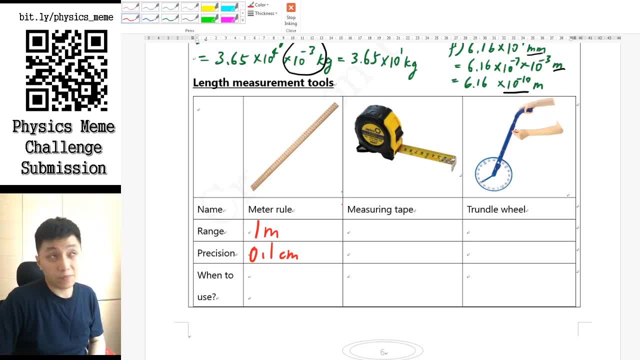 the thing is it may, simply may not be exactly six point seven cm. it could actually be six point seven, 2 cm, but with such a ruler there's no way I can know that it is six point seven two. I can only say 0.8, at most right in between 0.7 or 0.6 or 0.8, but i can't say it's 6.72. okay, so that means. 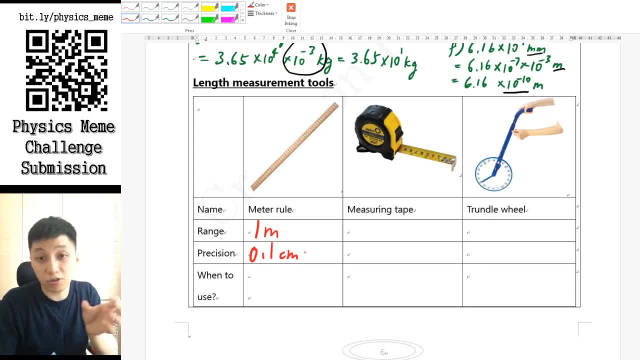 this limitation is, i mean the precision showing us the limitation of your tool, and that's very important in physics. as for the time when we will use it, i would say, uh, for most of the time when we measure object, of course, that is within one meter, first of all, and also, um, really some more. 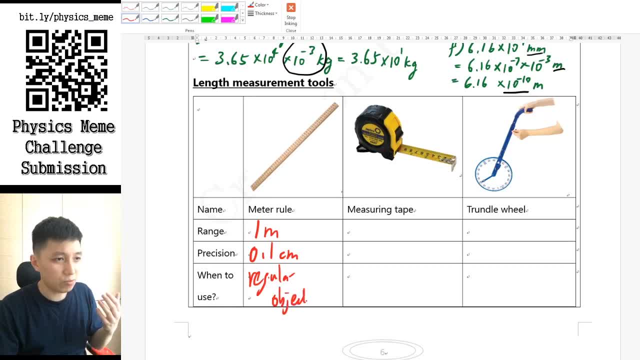 regular object because, um, this is more like using for measuring a certain distance when in your experiment, or the distance of a string, etc. so for things like that are rounded or much longer, then you obviously cannot use a meter ruler to measure. so for the other two questions, i'll leave it to you. now. please try it out. pause the video. 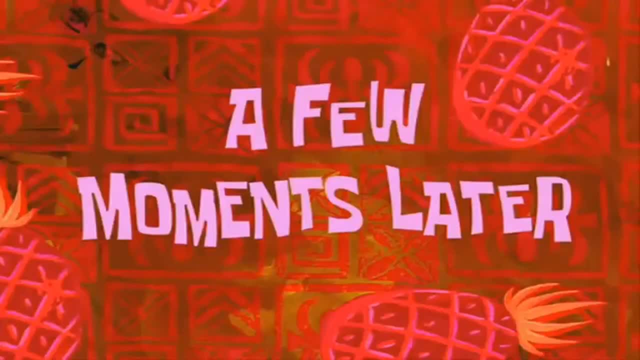 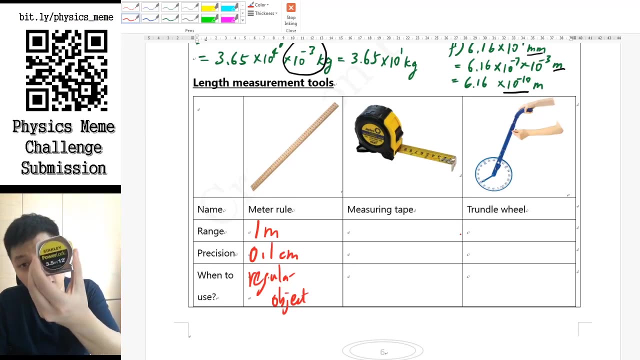 continue the video after you finish it a few moments later. all right, let's talk about the measuring tape first. so i happen to have a measuring tape at home. actually, i think it's quite common that you have one at home. just ask your parents, probably you can find one. 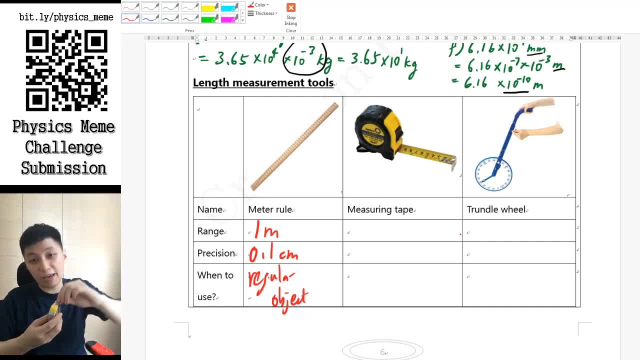 so, uh, i guess you have used it. just pour it out. and you know, just be careful with your fingers sometimes, or your eyes as well, when you use it. you can also use it as a measuring tape or lock it, and then it will just stay there, right? probably you have used it in detail lesson too. 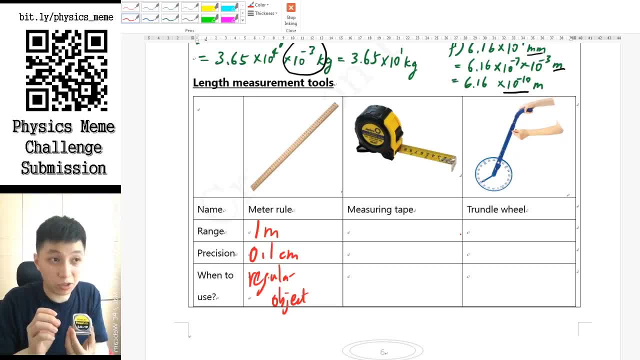 so the most important thing in physics here is: we want to know about its range. in fact, for each different measuring tape is different depending, depending on the model. so for mine, you can see here it's written as a 3.5 meter. so i'll trust it. i mean, i can. i can actually. 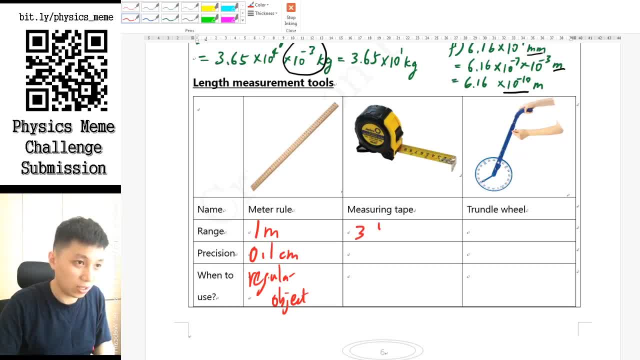 pull it out and check, but then i guess, uh, i will just check it, so i'll put down 3.5 meter. if you have a different one, i think that's fine, but usually for these it will probably between three to four meter or even longer, but then, uh, i don't think it can be too long because, uh, in that case, 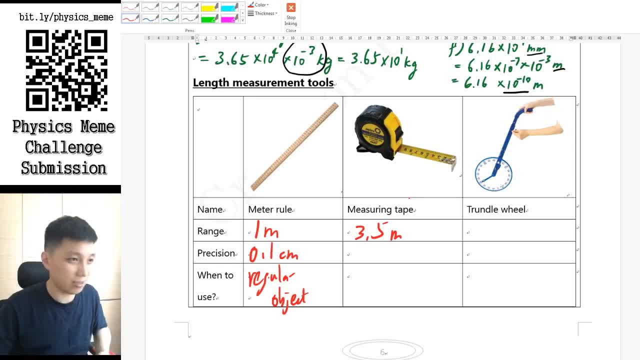 then you can. you can imagine this will be much bigger and that's not handy enough. so around three to four meters, i think. as for precision, let's take a look together. um, they actually provide both inch and also, uh, cm. so, uh, you can see that it is the same as the normal ruler that we use, like the. 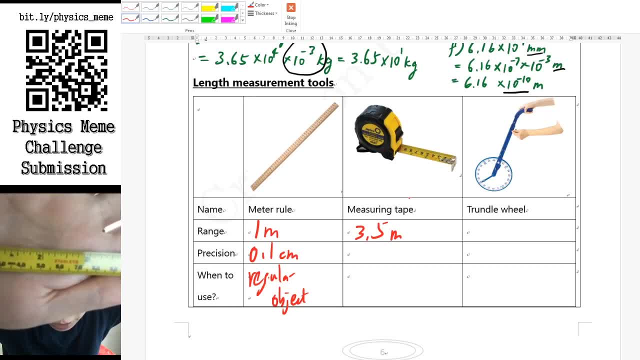 meter ruler that we just showed earlier that in between the two cm, the lower row is the cm, the upper row is for inch. so we will just stick with si units. so inch is not going to be used in physics basically. so for cm, uh, you can see there. 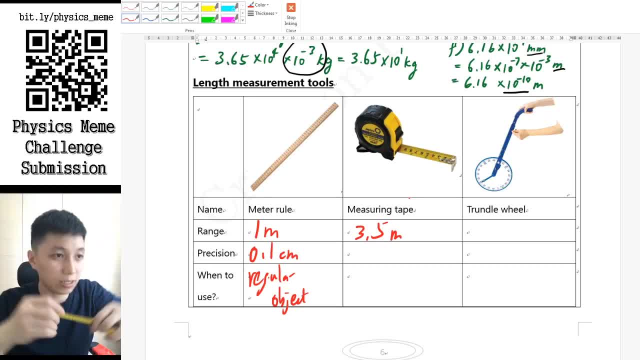 are 10 division or 10 intervals between them. so once again, uh, it is the same as a meter ruler, so i would say 0.1 cm again. so unless you have somehow a more precise one, in fact, for a ruler, i did own a ruler, but it is somehow lost. uh, that is more like a metal ruler manufactured. 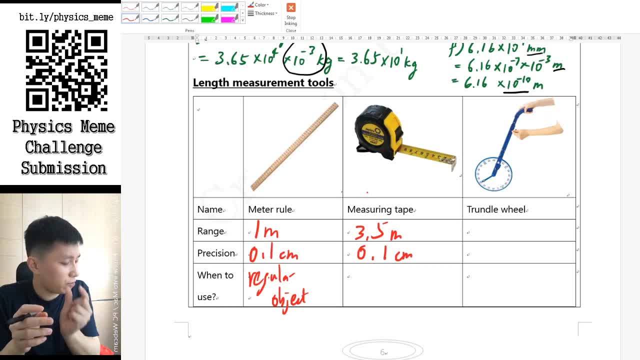 by i don't know what company, but then, uh, the first very few cm, like 3 cm. they also provide even smaller, so it's probably like, uh, i don't know, 0.01 maybe i, i'm not sure. but then uh, yeah, it actually is really different from different models. and then this: we are talking about the most general case. 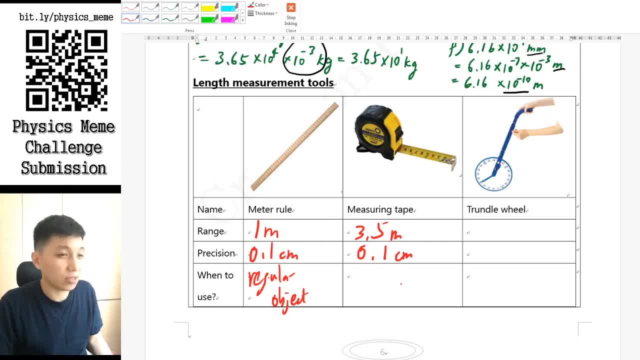 for the time when you will be using measuring tape, obviously, is when you uh don't have, you know, enough length for meter ruler, as in maybe something that is, uh say, the length, uh, the height of a door. um then, yeah, usually it's around around two meter roughly. so then, using a meter ruler, 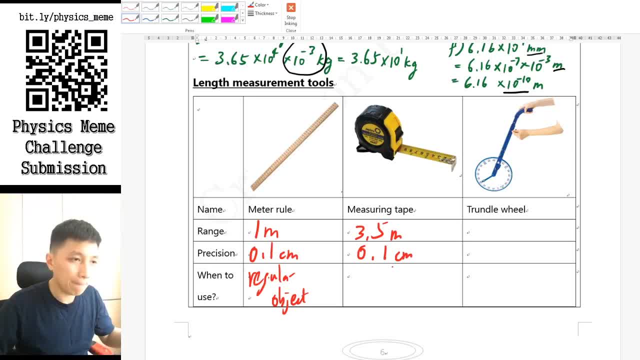 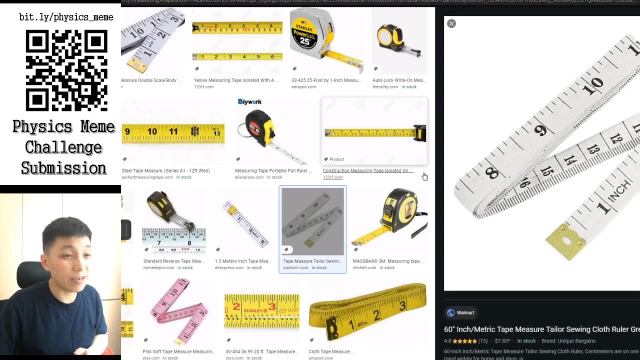 would not be able to help you um. at the same time, you may also, you should also realize that for measuring tape- in fact it is not just limited to the one that i'm showing you right now- uh, there are some sort of tape measure people may call. 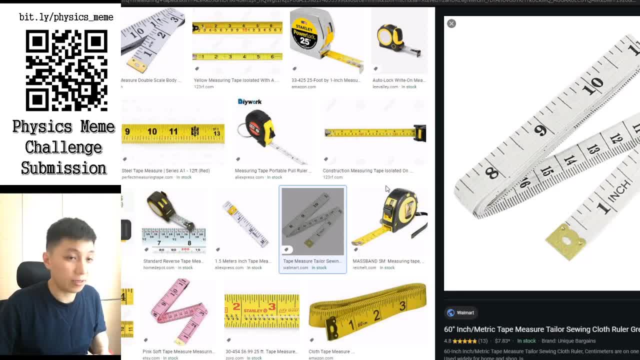 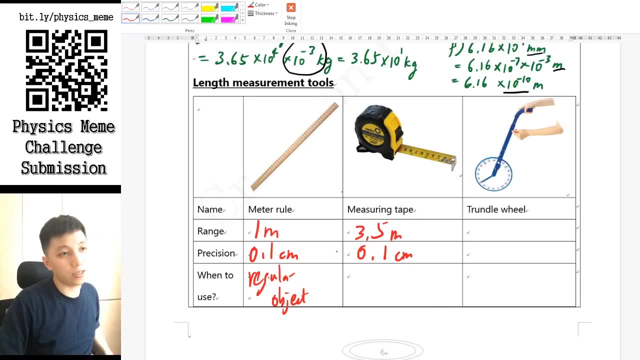 that is soft for maybe textile tailor for measuring. maybe when you're trying to make some clothes you know you want to measure your body size, then you need to use that so for some sort of measuring tape you can actually use for rounded object. so both, I will say both regular and rounded. 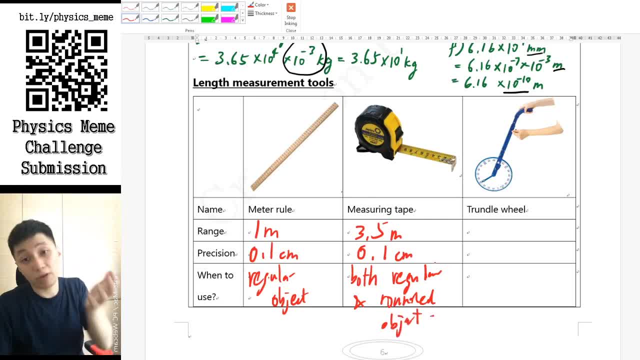 object. all right, depending on. I mean, if you have a software, then you can do for rounded object, of course. lastly, for the wheel, we actually- I mean people just call it wheel usually, but then the proper name could be called as trundle wheel. all right, I don't know why it's called trundle. 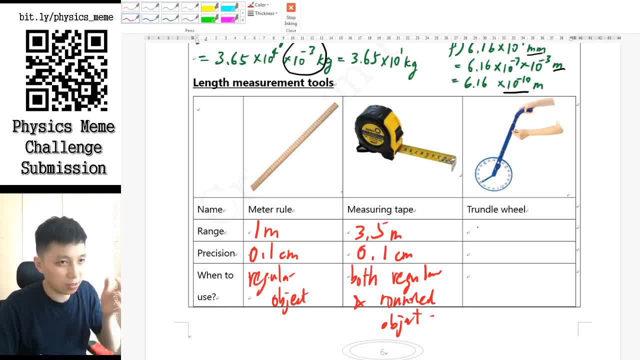 wheel, or maybe it's. if someone, anyone know, let me know in the comment section. but then this is the name. and if you apparently don't have it at home, but then you can imagine, when you try to use it it will be keep turning and usually there's a click sound whenever you pass through a certain 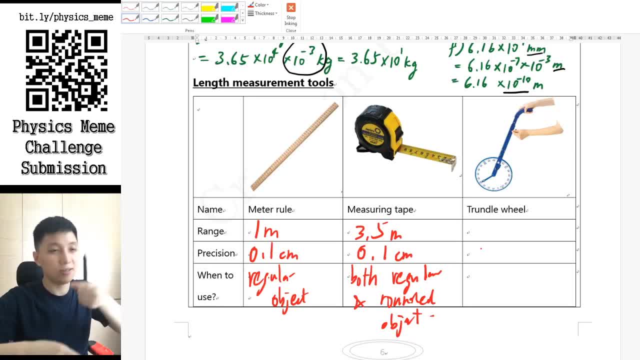 point, which is click, click, click, all right, and each click sound. most of the models I've seen is one meter, so whenever you just measure a certain distance, you just kind of roll over it. usually it's the grind, simply, and then you can count by listening, hearing how many clicks that you're producing. so for the range in, 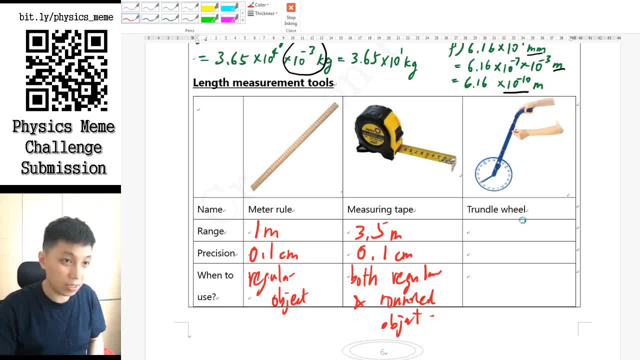 fact, you can keep going: right, it's actually infinite. so I would say it's actually infinity. okay, and for the precision, again, it depends on how you do it. if you only count on the click sound, that means I just keep rolling and then I find out: okay, click, click, click. 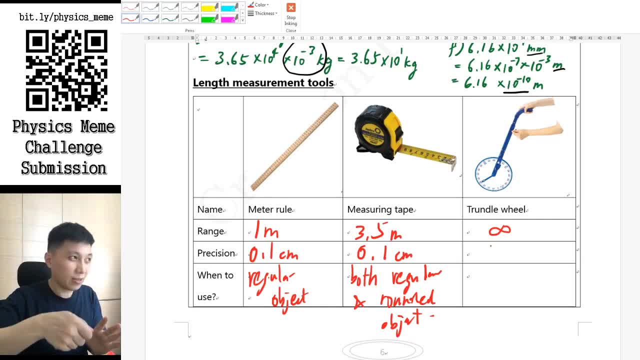 five, say five times, all right, and then I keep going a bit up to the destination. I want to stop. I don't have the sixth click, so that means it's in between five meter to six meter. okay, so if you are only doing in this way, then obviously the precision is only in one meter, or you can. 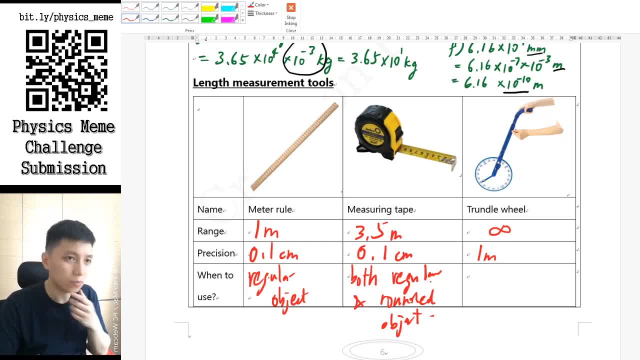 claim half of it. so 0.5 meter- that's one way of doing it, or if you can ensure that your starting point is actually zero meter and they keep going up. after the five click and then you kind of see: oh, it's almost the end already, so you keep going, and then you see the. when you stop the wheel, you